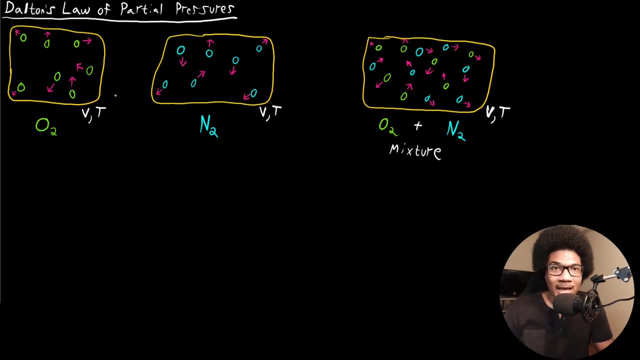 and N2 gas. here They're in the same container, that's of the same size and at the same temperature right. So in each one there's a volume V, a temperature T, right For each of these samples of O2 and N2.. And when we mix them together in a container of the same volume and 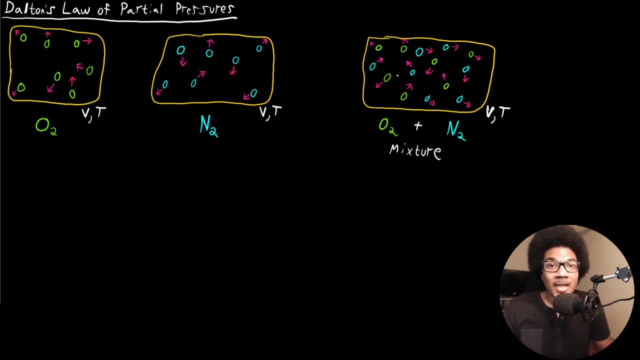 temperature right. Each one would exert the same pressure in the mixture that it would by itself. So it's basically saying that each individual gas is more or less agnostic of the other. gas is in the mixture right. It's going to exert the same pressure, whether it's in that container by 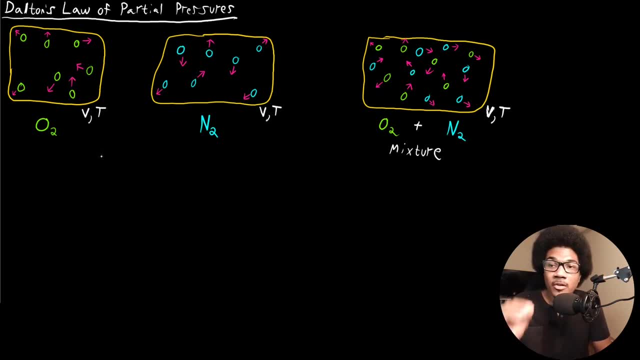 itself, or whether it's in that container, in a mixture. So what that allows us to do: if we want to calculate the pressure of this gas mixture of O2 and N2, right, We'll have a total pressure which I'll call P total. This is the total pressure of the mixture. What we can do: 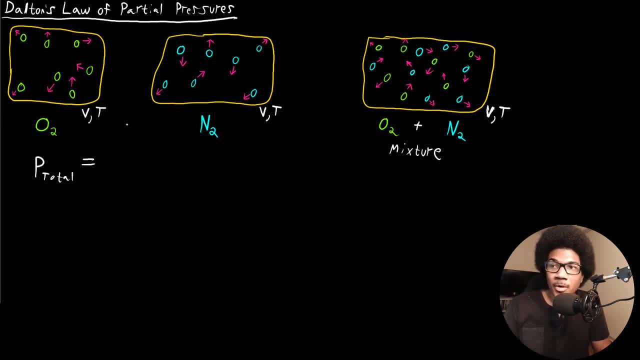 is just sum up the partial pressures of each of these gases, Right? So we'll call the pressure that the gas exerts by itself. It's partial pressure, And you just sum up those partial pressures for each individual component in your mixture. So if this: 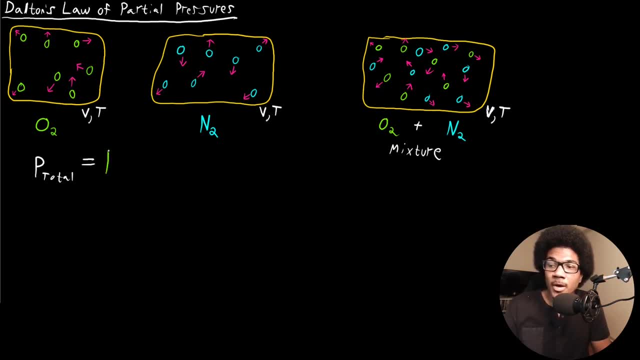 is a two component mixture with O2 and N2, we'll have a partial pressure for O2. And we just add on our partial pressure for N2.. Right, So this would give us the total pressure of the mixture as just a sum of each of the. 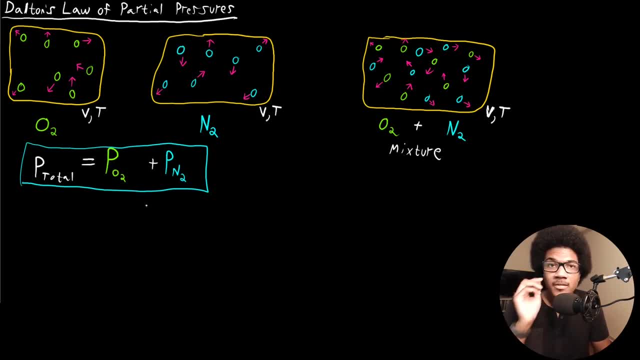 individual partial pressures of the components in that mixture. And again, the partial pressure is just the pressure that that gas would exert if it was in that container by itself. right, That's going to be the partial pressure of that gas. So you sum up both of the partial pressures you get. 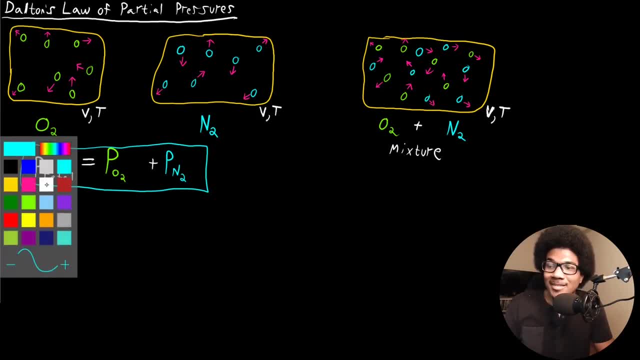 the total pressure And obviously this could be extended to the total pressure of the gas. So if you can just calculate that, if there's a multiple plus or one compared to cases where there are more than two components, right, So we can calculate P stations. 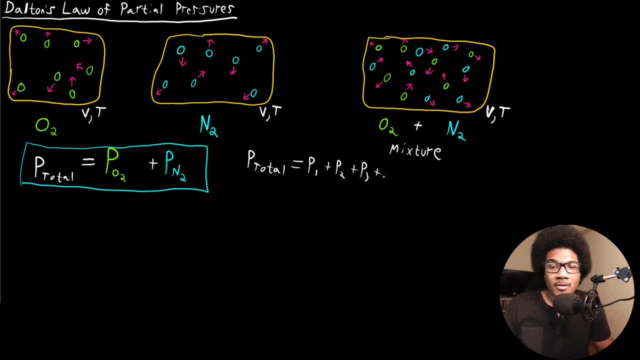 for many components, right. So it will just be p1 plus P2, plus p3, right? dot dot dot. however many gases you have in a mixture. If you've got 100 gases, just add up the hundred partial pressures in. 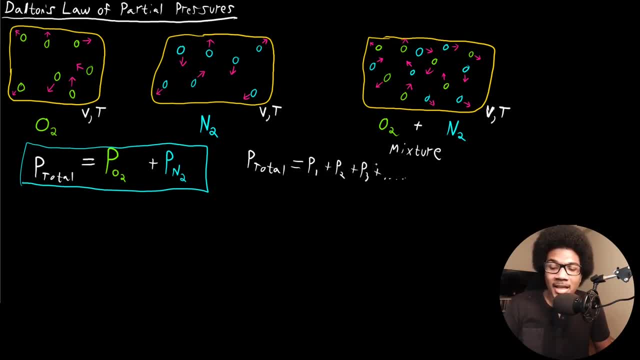 that mixture: right? So you just keep adding on the different partial pressures. gas mixture: right? so this is the total uh pressure of the gas, and then all of these would be the partial pressures. you're just summing up the partial pressures for the gas mixture. now we can. 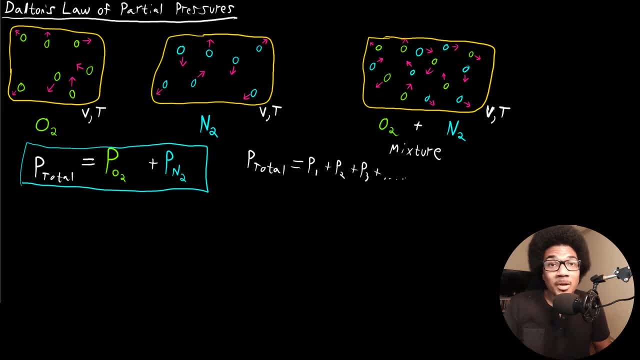 actually solve for each of these individual partial pressures. if we assume that the gases are ideal- right. so if we assume an ideal gas, so assume ideal gas- then each of these partial pressures can be calculated explicitly, right. so, for example, p1 would just be equal to the number of moles of that first component of the gas. 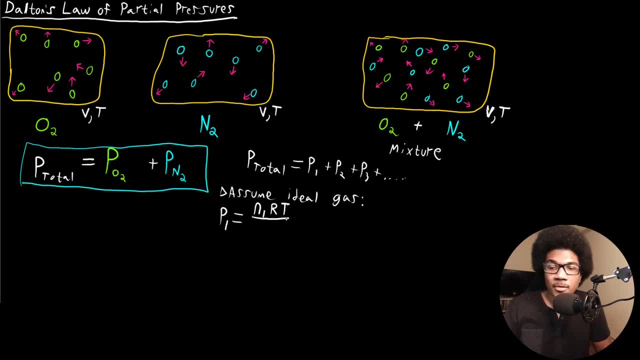 times the gas constant temperature and the volume. keep in mind that the temperature and volume are going to be the same for each component, right? they're in the same container, so the volume and temperature are going to be exactly the same. we can write out an expression similar to that for: 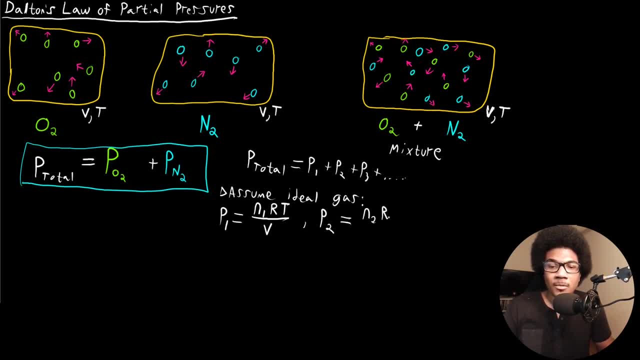 p2p right. so you got: p2 is going to be equal to n2 rt over v, right. we can get an expression for p3 right. p3 is equal to n3 rt over v, right. the only thing that's changing is the number of moles of your. 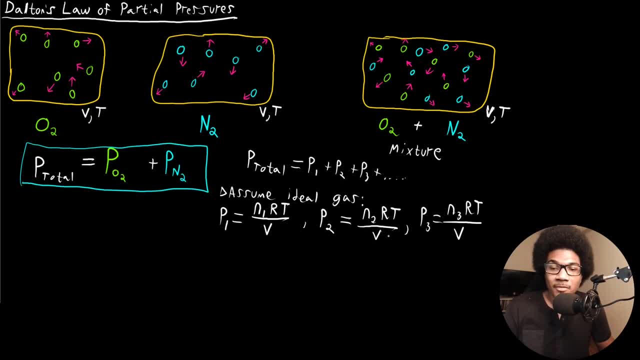 component, right? uh, everything else is the same. temperature is the same, volume is the same, and you would just get a different partial pressure for each individual gas. and obviously you can do this on and on and on for each component in your mixture, right? so if we assume that the partial 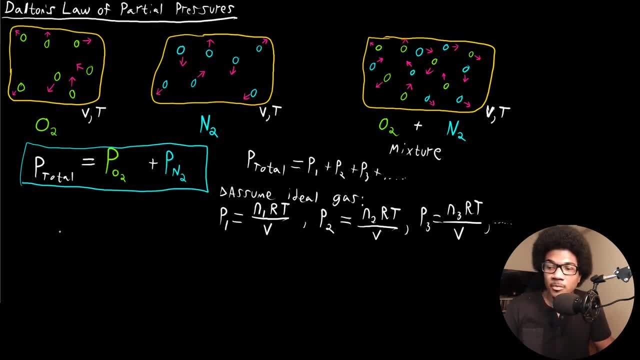 temperature is equal to n2 rt over v, right, then we can just write out an expression for p1, right? so that means that we can re-express this p total expression, right. so p total, it's going to be equal to right. if we plug in p1, right, we got n1 rt over v, plus in two rt over v. 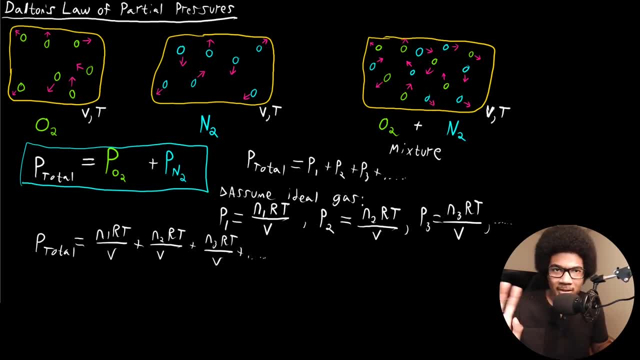 right plus in three rt over v right plus dot, dot, dot, however many uh components you have in your gas, right? so the only thing that's changing here is the number of moles. so we can factor out rt over v, right? so we got rt over v, and the only thing that's different here is the number of moles. so 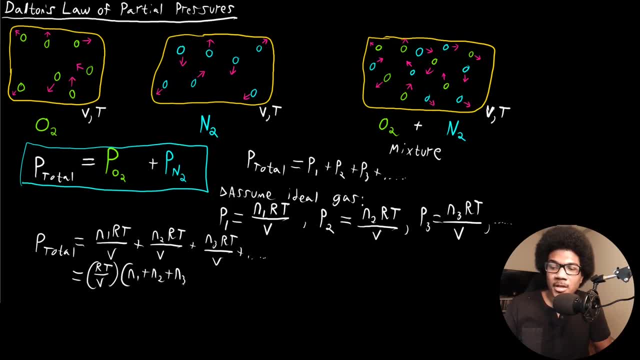 we got n1 plus n2 plus n3 plus dot, dot, dot, right. so that's p total, right. so the only thing we need to know is the number of moles of each component um in order to solve for this right. so we need to know the total pressure, right? so this, in this sum of the number of moles, is: 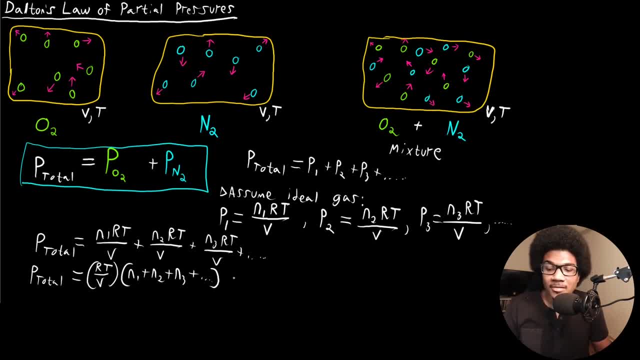 going to be the total sum of the number of moles of your gas gases in the mixture. so we can express p total right, our total pressure for our mixture, as n total times rt over v right, where n total is just your um, where n total is just your total number of moles of all the molecules. 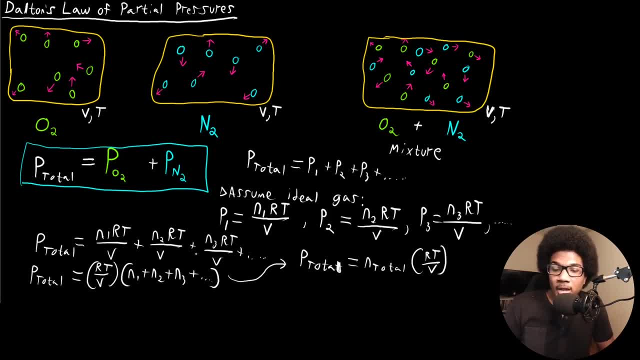 of the gas components in your mixture right. okay, so we know that we can solve for each of these partial pressures using the ideal gas law. we know we can sum them all up to get the total pressure right. this is dalton's law of partial pressures. let's look at an example problem to to bring this: 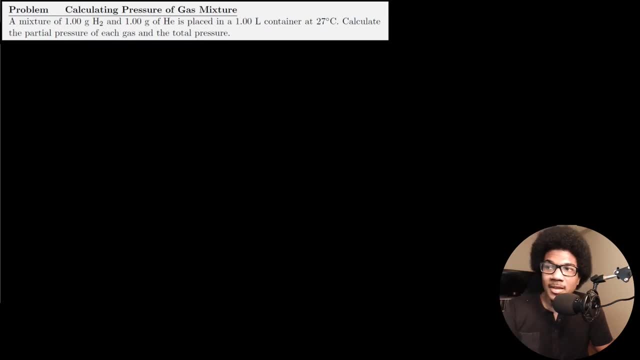 home. okay. so this problem says a mixture of one gram of h2 and one gram of helium gases are placed in a one liter container at 27 degrees c. calculate the partial pressure of each gas and the total pressure, right? so we've been given two different amounts, one of uh- hydrogen- and one 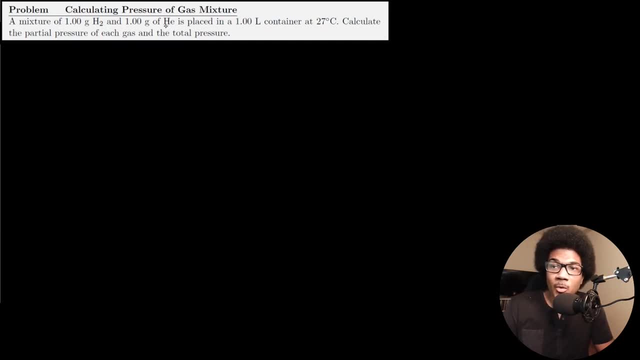 of helium, right, one gram of each gas, and we're asked to calculate the partial pressure for each gas and the total pressure, right? so let's? let's think about what we've been given here and what strategy we can take to solve this problem. so we've been given 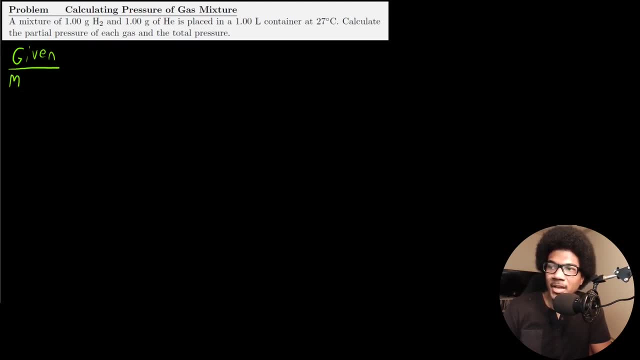 you right, we've been given the mass of h2, so i'll use m sub h2. we got one gram of h2. we also know we got one gram of helium. okay, so one gram for both of those guys, right the volume: we've also been given one liter and we've also been given the temperature, right. and since we've 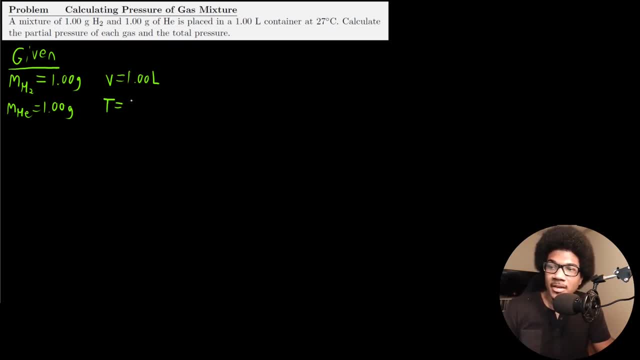 we've been converting each of these to kelvin, so i'm just going to go ahead and write this in kelvin, so that temperature is 300, 0.15 kelvin. right, that's what you get if you convert 27 degrees c to um to kelvin. okay, so this: 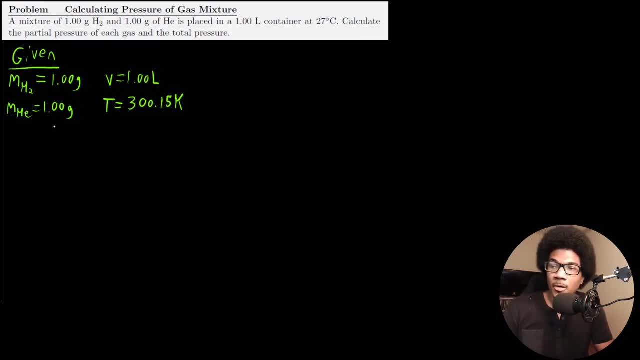 is what we've been given. now we just need to solve for the- uh, the partial pressure of each gas. what we're going to need is to convert these masses to the number of moles of each of our component in the mix, each of our components in the mixture, right? so let's do that, so we know we have one gram. 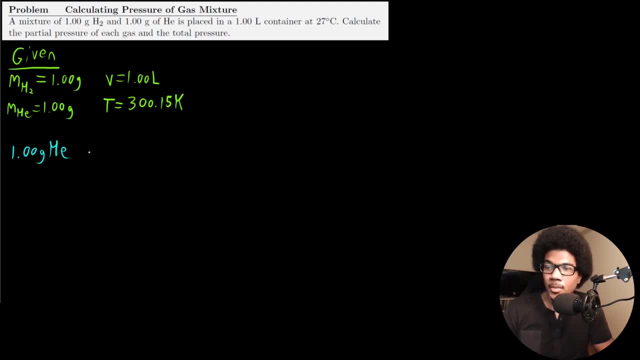 of helium, of helium, and the molar mass for helium is 4 grams of helium for every one mole of helium, and so that's going to give us 0.25 moles of helium. that is in our gas mixture. right, we have one gram. we convert that to moles. we know we have 0.25 moles of helium. now we also 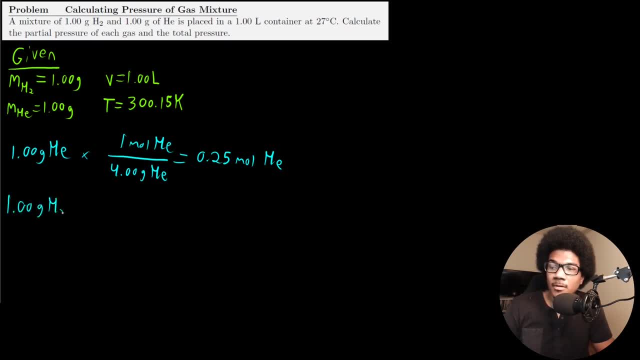 have one gram of h2, right? so we got one gram of h2. for every one mole of h2, there's 2.02 grams of h2. so, um, using that right, we get about 0.5 moles of h2, right? so we've converted both of our uh. 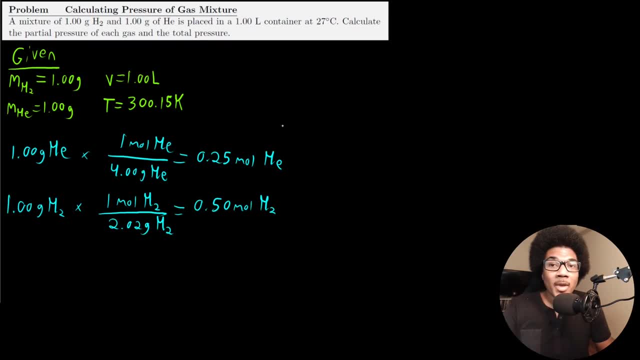 both of our masses, that we were given two moles. now we have everything we need to calculate the partial pressure of each gas. so let's plug in, so we have the ideal gas law. we know that our we can calculate our partial pressure for h2. let's do h2 first, so the partial pressure for h2 is going to. 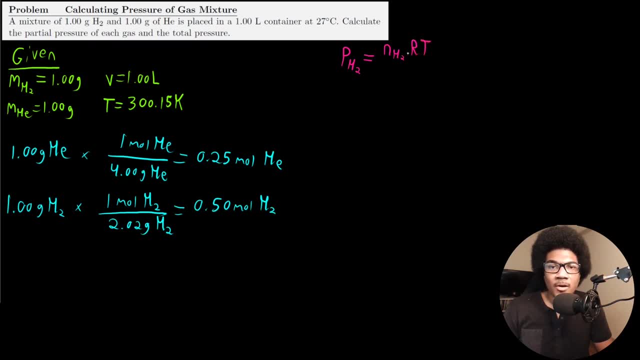 be the number of moles of h2 times rt over v, right, we just calculated the number of moles of h2, that's this 0.5 moles. so we can plug that guy in, right? so we got 0.5 moles of h2, our gas constant. 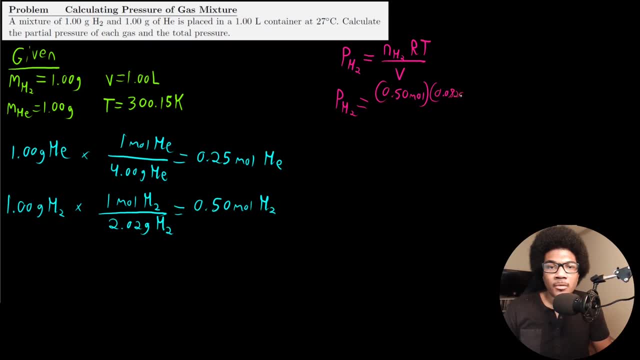 0.08206 liter atm per mole per kelvin. right, our temperature here is going to be 300.15 kelvin and the volume is one liter. so we put that in the denominator. so we got one liter for our volume. so our partial pressure. first let's check our units, right. so looking at our units, 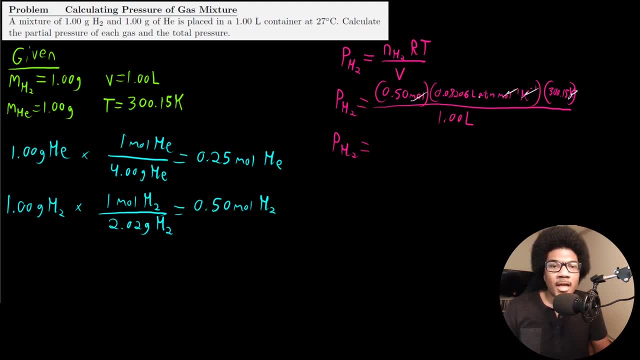 moles cancels out here, kelvin cancels and liters cancel, so we're left with atm, which makes sense, since we're trying to calculate a pressure, and so for h2 our partial pressure is going to be 12.31 atm right now. using the exact same procedure, we can calculate the partial pressure for: 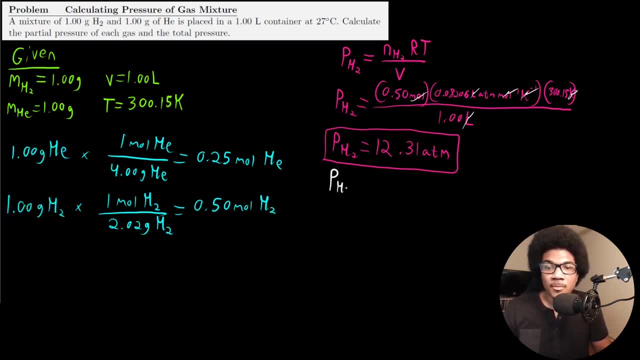 helium, and so if we use that same procedure- i'm not going to go through the calculation, but you use that exact same procedure- then you get the partial pressure for helium, which is 6.16 atm. okay, so we've got our partial pressures for both h2 and h2. so we're going to go through the calculation for the partial pressure for the helium and 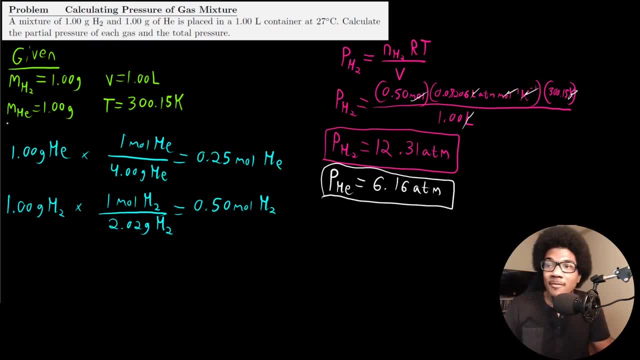 hydrogen and helium in this mixture. now we have everything we need to solve for the total pressure of the mixture, right. so to solve for p total, right, we have to do the partial pressure of h2, according to dalton's law, plus the partial pressure of helium, right? so if we add those two numbers together, there's 12.31 plus the 6.16. 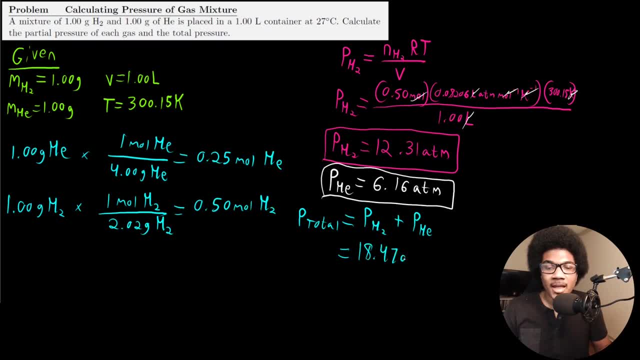 we get 18.47 atm as our total pressure for the mixture right. so that gives us our p total right. so, as you can see, you can use dalton's law- uh, using that with the ideal gas law, right, we can use dalton's law in order to calculate partial pressures and then just sum them all up, uh, to get. the total pressure of a gas mixture right? so if we add those two numbers together, we get the total pressure of a gas mixture.